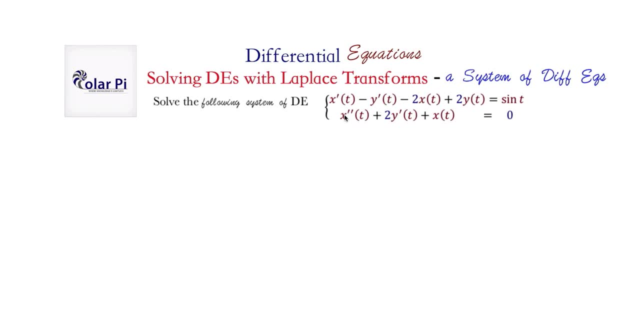 a system we're going to have two functions, right, Like remember, uh, in those three examples, uh, and each of them, even in the one that was a fourth order, it was just one function, It was Y and its derivatives. But here we have Y and its derivatives and X and its derivatives. 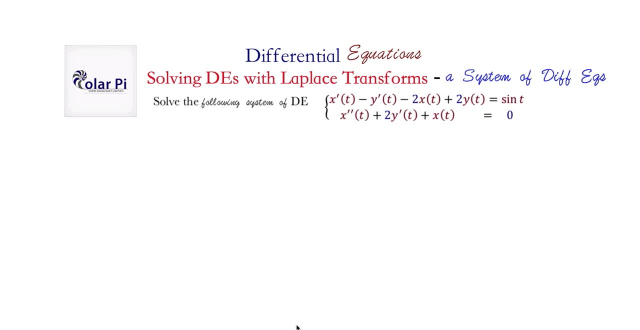 and therefore a system right. Okay, Therefore, uh, to start, we need to define not just the Laplace transform of Y, but also the Laplace transform of um X, right And uh, for reasons I mentioned, uh there in that first video. 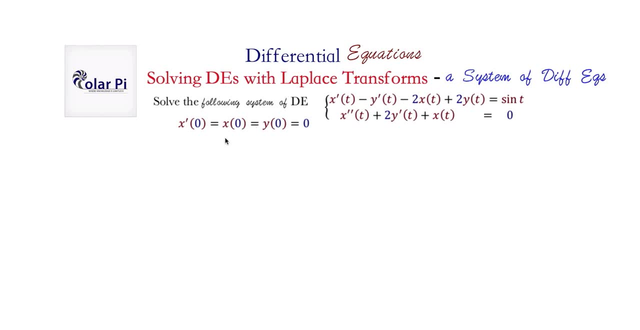 on solving differential equations with Laplace transforms three examples, right, Remember? Yeah, So there, um, I mentioned why uh, the initial um value uh has to be given, for T equals zero, And so I'm not going to say it here, I'm going to incentivize watching that video. Um right, Um. 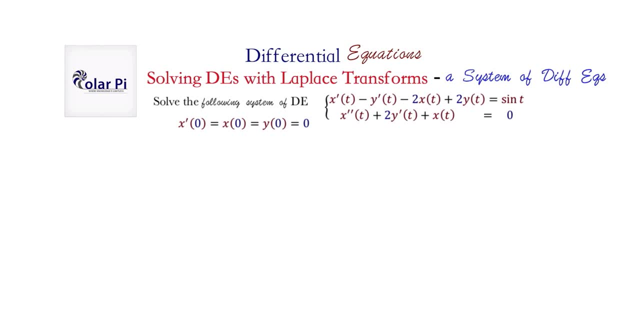 in case you're dying in curiosity, and, um, in case you can live with it. well, let's test your result. Um, all right, All right, But yeah, as I said to start, we need to define: uh, both the. 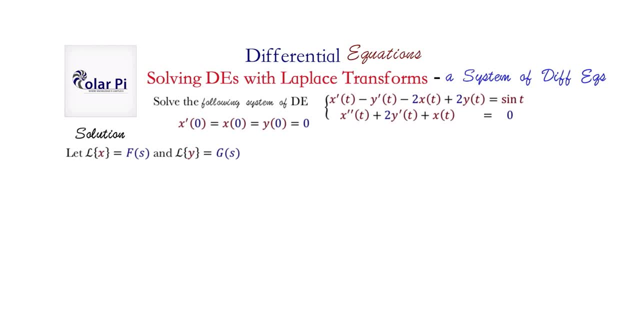 Laplace transform for the function X and the function Y, And I suppose, for a reason that has to do with the fact that X comes before Y, And so I'm not going to say it here, I'm going to say it for Y. as um F comes before G, We've chosen to name them in this manner. right, Uh, but otherwise. 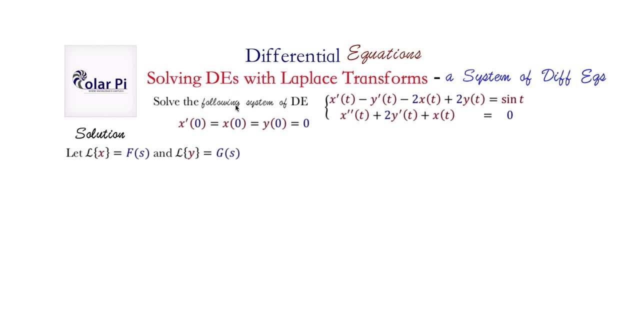 you know, just as I said there in that first video, it's nice to have handy, uh, the formula for the Laplace transform of uh Y prime and the formula for the Laplace transform of Y double prime, Y prime, Y double prime or X prime, X double prime or X double prime. So uh, 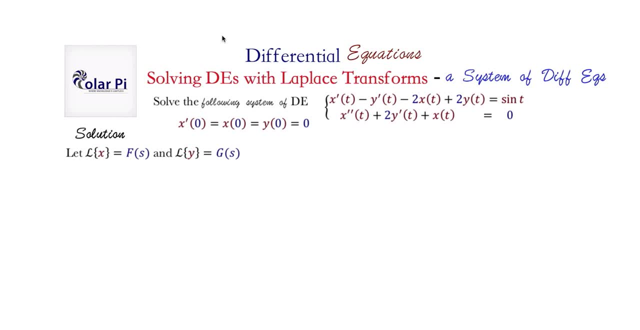 F prime, F, double prime. doesn't matter how you write it, but it's nice to have those uh formulas that I had um shared with you there in that first video. uh, with the three examples right And of course, those formulas uh for the Laplace transform of um, Y prime and Y double. 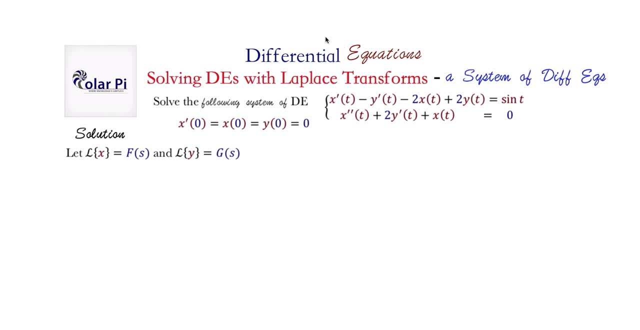 prime. uh, both of those I dedicated videos to and I showed you how to derive, in two separate videos, uh, both of those formulas in their own individual videos. So, uh, I'm going to show you so you can check those out for more details. but yeah, because I already, like you know, 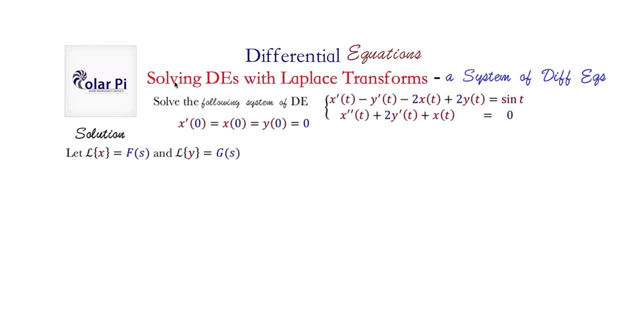 like, walked you through uh, the formulas carefully there in that first video. I'm not going to do it as much here, And you should also know that, uh, the next thing we're going to do is take the Laplace transform of, uh, both sides of this first equation and do the same with both. 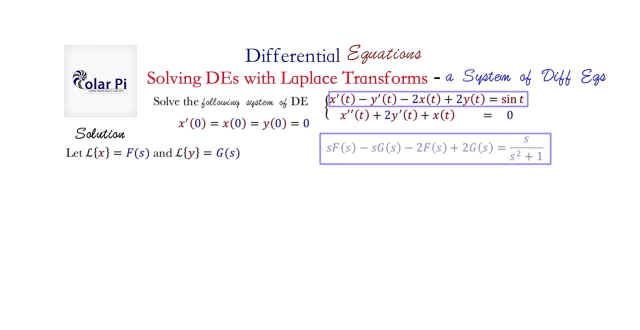 sides of this second equation, And so, uh, we get on with that Um and uh. for the first uh equation, it's going to turn out to be Y prime. So, uh, I'm going to show you how to derive. 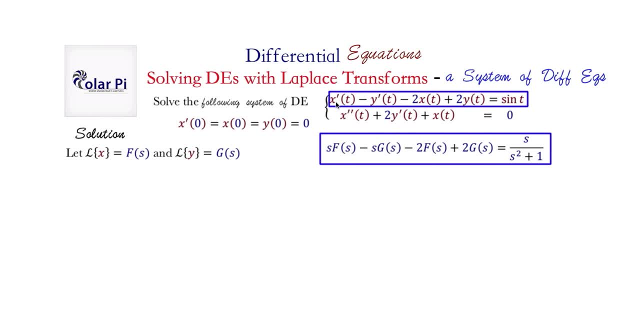 and very quickly. quick reminder is that, like the Laplace transform for um X prime, for example, is going to be S times capital F of S, because yeah, And then it's going to be minus um X of zero, but X of zero is zero, And that's why you don't see minus zero here, And uh, you get it. 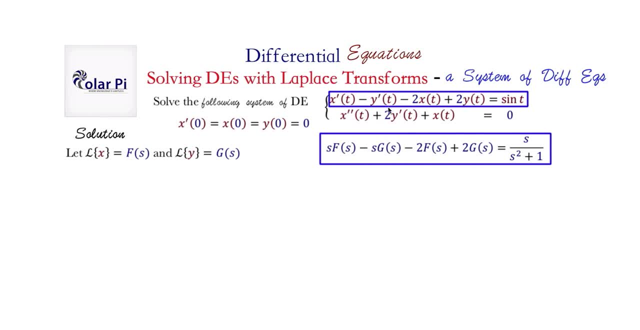 get it. get it Okay. Otherwise, um, yeah, for uh this you need uh minus uh Y of zero in this part. but Y of zero is also zero, And that's why you don't see it. 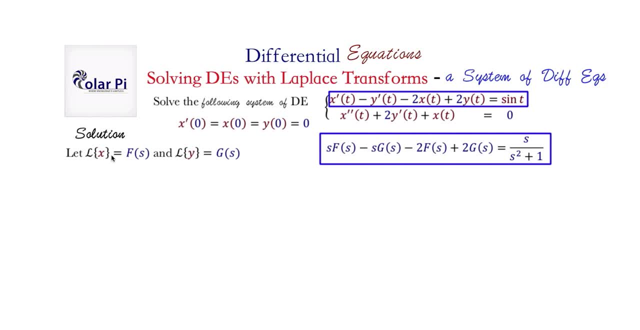 Otherwise, you know, this here is that by definition and this here is that, uh, by definition. But yeah, what I've said very quickly, if you missed it, is that, like, I did apply that formula for the Laplace transform of the derivative both in this part and this part. It's just that like 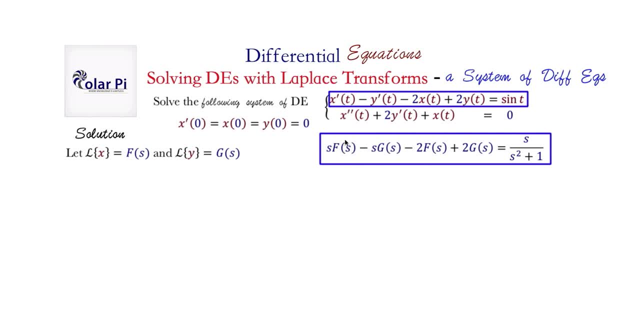 um, these two guys which would have been subtracted from this and this respectively, are both going to be Y of zero. So, uh, Y of zero is also zero, And that's why you don't see it. So, uh, Y of zero is also zero, which is why you don't see them there. Yeah, Okay, Otherwise, 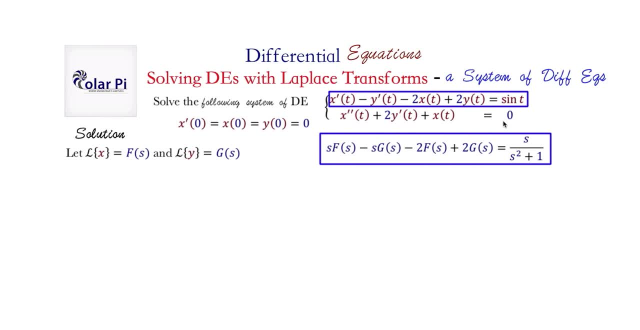 you know, we need to know the Laplace transform of sine and uh, basic things like that. And so that's that for the first equation. but uh, we can make it more convenient this first equation by grouping the capital F's and the capital G's And um, so if we do that then we can write it. 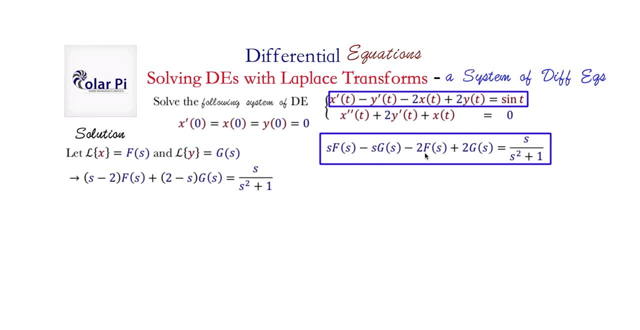 a bit more succinctly, if you want to call it that in this manner: right, Like, okay, And so, like you know, we've paired these two and then taken out, um, I'm taking out uh a G, a G from um, uh, them pair these two, right, And then them pair. 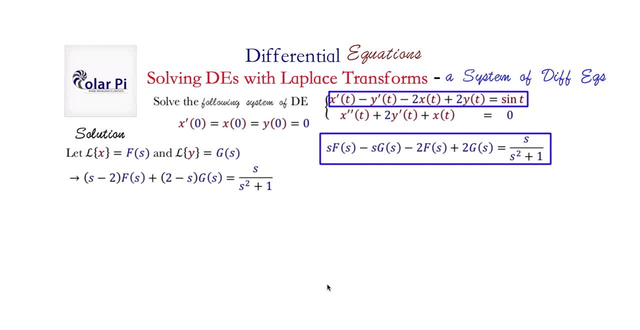 we've taken out an F from right, Capital F. Yeah, You get it. You get it. It's basic algebra. Like I shouldn't uh have to walk you through that like too carefully. Okay, Now, um, yeah, Right. 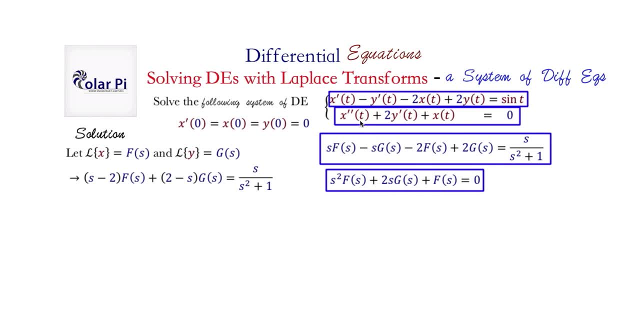 Like and um. okay, So clearly we've uh applied the formula for the Laplace transform of the second derivative and uh also for the Laplace transform of the second derivative, And uh also for the first derivative, but obviously a second derivative of X and a first derivative of Y, And uh the 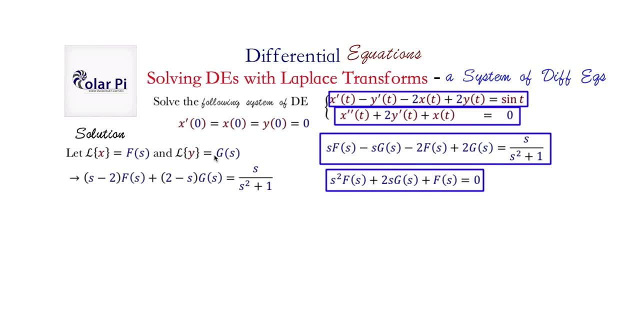 impact there is, obviously, whether um capital F is involved in, uh, capital G G's involved, and they are involved where they need to be- And um. this too, we could write a bit more conveniently: um, uh, like this: And so now we have, like our system, uh, translated in terms of Laplace. 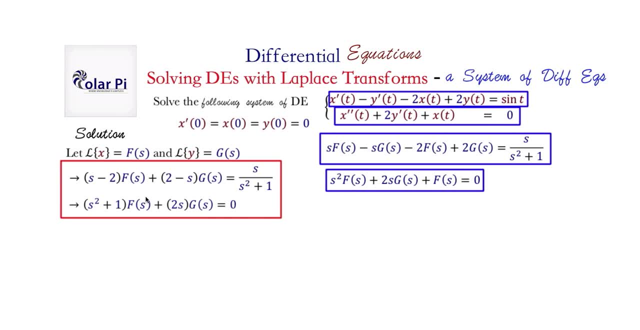 transforms, But still just a system. I noticed that this is this is a system in two unknowns. The two unknowns are capital F and capital G And so, like you know, we've seen a system of equations in two unknowns. As long as we have two equations in the two unknowns, we can solve them, And there are a. 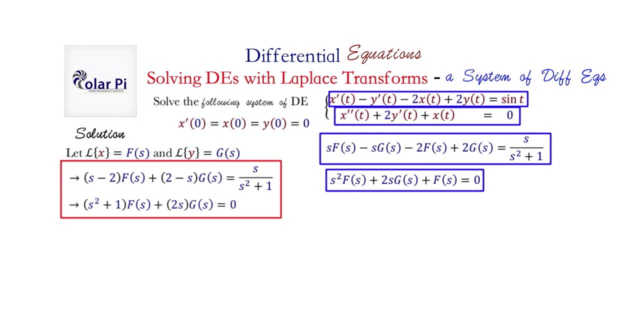 variety of uh ways, of ways of solving a system of two equations and two unknowns, And one of them is uh Kramer rule, And that's what I'm going to choose to use here, And I'm going to use this: 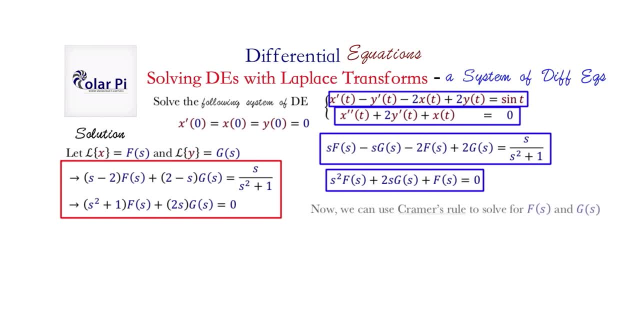 here and I have a video in my algebra, one videos dedicated to teaching you Kramer's rule. So I'm not going to talk about Kramer's rule details here. You can watch that video. Um. but yeah, um, first thing you need to do is, uh, find uh the determinant of the matrix of coefficients, where? 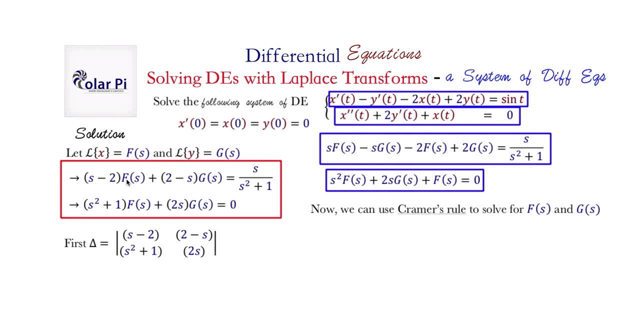 the coefficients here, in this case, are anything but capital F of S and capital G of S, And so, like you know, that's how, like the coefficient in this part, for example, is this the coefficient in this part, is this and uh, the coefficient in this part? And so this is, uh, the determinant of the matrix of. 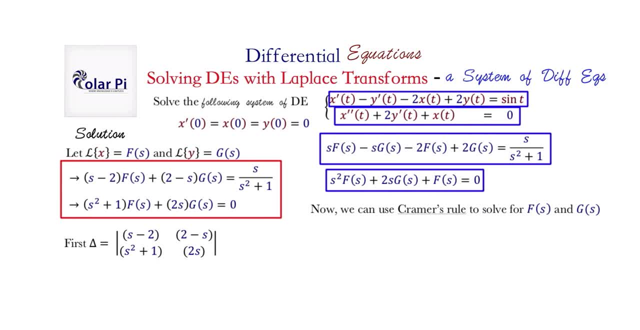 coefficients right And um. so that's one of the things that you need to do for Kramer's rule, And so, when we're um, solving for um, solving for um capital F, what we're going to need to. 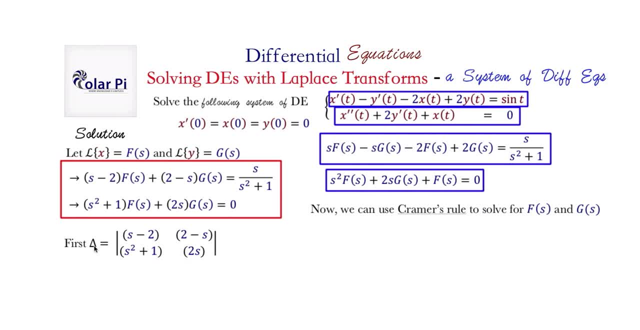 do in addition to this, uh, the determinant here which we've uh called Delta. In addition to this, what we need to do is also calculate, um, the determinant of a two by two matrix, uh, where it's almost like this: 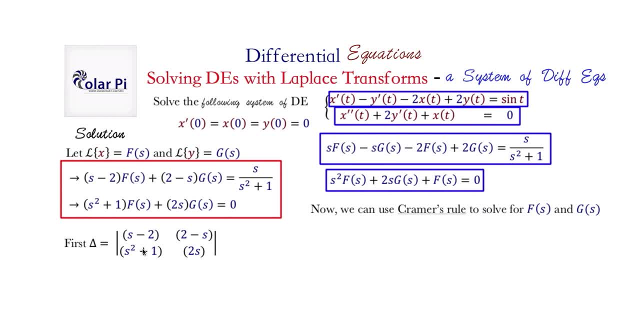 matrix, only for capital F. we replace this column with this here as a column, right For capital F, And then for capital G we take the same guy again, but for capital G. we replace this column uh with this taken as a column. but that's already telling you more details of um Kramer's. 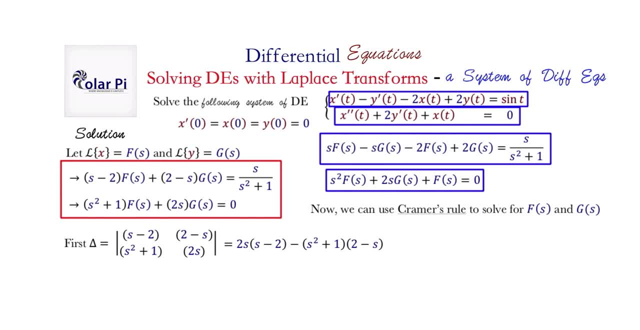 rule than um. I should, just so that you know you're not like totally lost in what remains of this video. but like, yeah, like, as I said, I have a video dedicated to Kramer's rule, So check that out. Um, but yeah, um, two by two determinants: I have at least a couple of videos on those, And 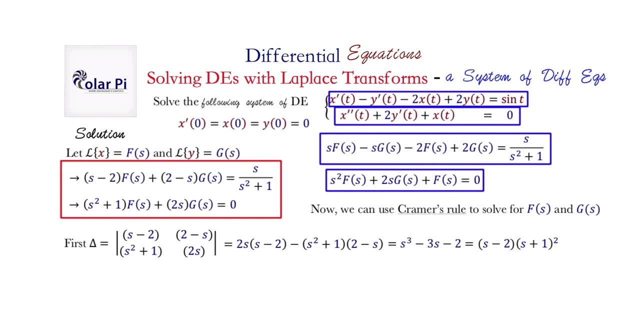 um, this is how that goes. Um, there's a little bit more algebra to do to make it nicer, So we do that right now. Delta: this here is the determinant of the matrix of coefficients. right there, Right, Okay, Uh, and, as I said, this is not the only determinant you need to do. 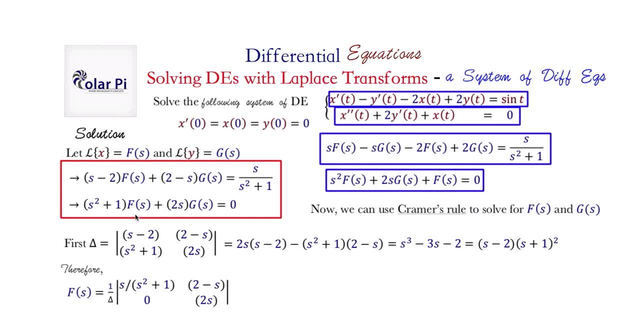 in order for you to find um capital F of S via Kramer's rule, You need to: uh take the uh determinant of uh, the matrix of coefficients, right, And so basically take this and put it in the denominator of the matrix of coefficients, Right, And so basically take this and put it in. 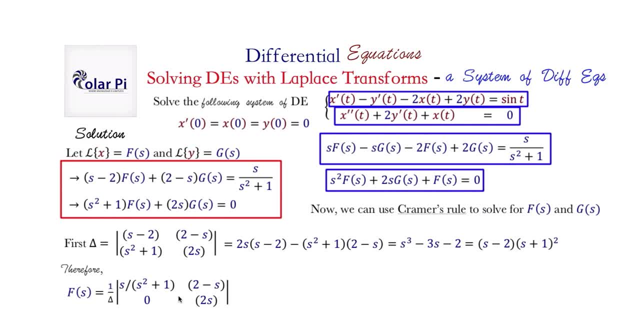 the denominator of the matrix of coefficients, right, And so basically take this and put it in the denominator and in the numerator will be the determinant of the two by two matrix, where um- as I revealed more than I should- for capital F. you replaced this column, which is this here with 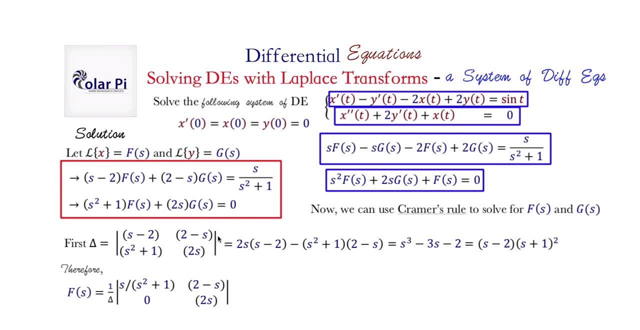 this taken as a column. And for capital G, you replace this column with this taken as a column. Since here we're doing it for F, we're replacing this here with that taken as a column. And then, of course, these vertical bars mean determinant, So we need to calculate this determinant And 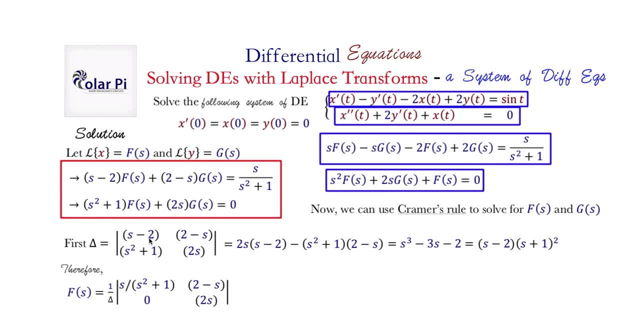 this is going to be the numerator where the denominator is Delta, this other determinant. Okay, All right, All right, All right. Again, I've um handheld you through, uh, Kramer's rule way more than I needed to. or shoulda, um, but shoulda, or whaddup, whatever right Let's. 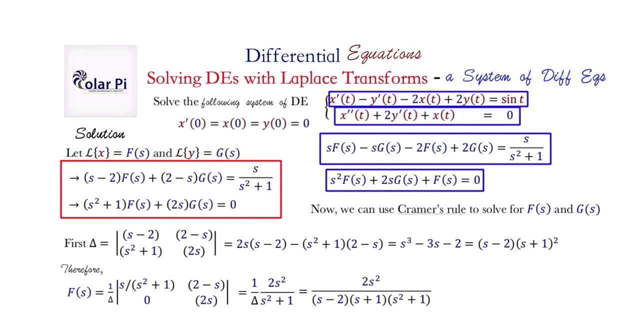 just finish. Um, all right. So, um, um, yeah, like, and so you get to this what I'm doing: it Over burning about this end, So, and then you can dump, you go chaos. That looks appropriate quality. 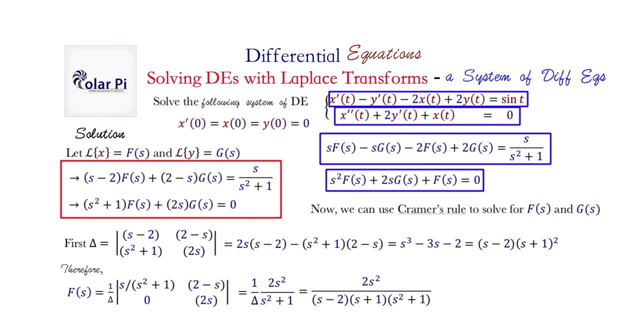 It sounds good. Okay, Um, what's good? And once we've captured it here, let's go over to our other drugs. and it. look at thearus called um across the physical general art. right, You could also use this to see, okay. 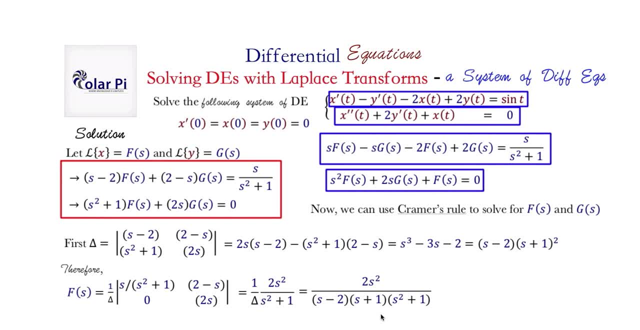 You know, it looks likeaczego we're hitting um red zone where, in your writing, um yeah, like, and so you get to this spot right, and so you're like: oh yeah, where to from here? uh, more fun. and that for you means partial fraction decomposition, uh, but for me it means 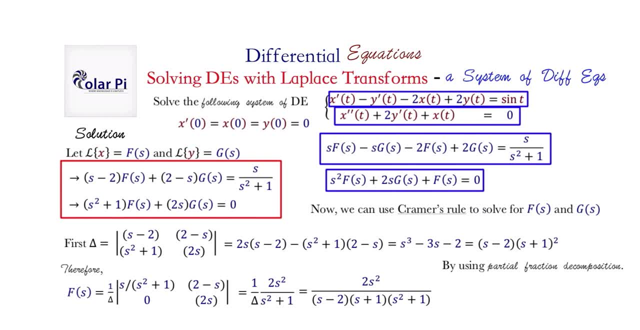 that i already know partial fraction decomposition, so i'm gonna, uh, skip that detail, and this ain't homework for me. i'm just like giving you free fun math lessons, and so there that goes. and um, yeah, so by using partial fraction decomposition- by that i mean doing lots of fun um computation. 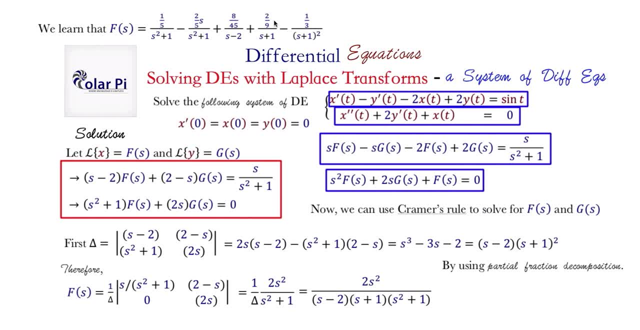 you show that this here is the same as this. i have lots of videos on partial fraction decomposition so you can check them out if you need to learn on that. but then otherwise you know, like, uh, easy recognition of inverse Laplace transforms of these individual guys will also go a long way, and that's the. 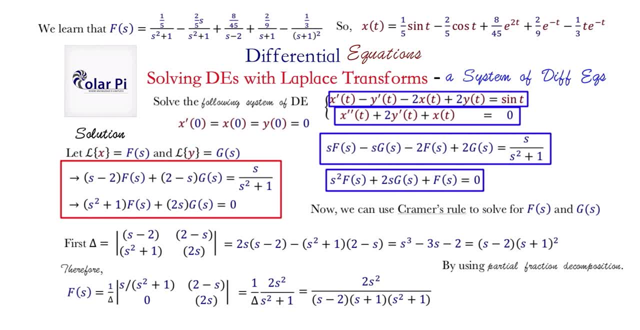 other um prerequisite to, like you know, solving differential equations with laplace transforms right and so like. for example, this here is like a fifth sine t and so on. right, like, so, like, yeah, like and yeah, and so only thing we have left to do to say we're done is we need to find capital. g. 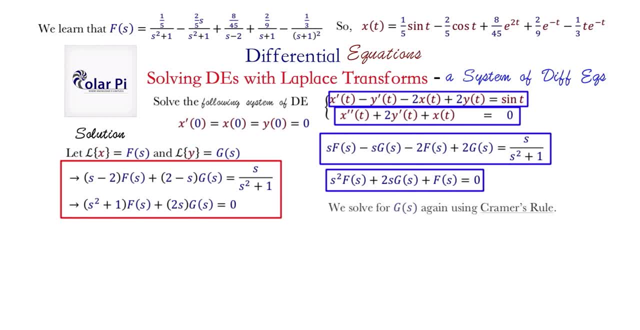 right and well, how does it go? i already told you kramer's rule. right like, and this time, what you're going to do is, uh, and that determinant that we had had here. you replace, as i said, the g columns with this and that's what you see. clearly, the f columns are unaltered. right like, because this time, 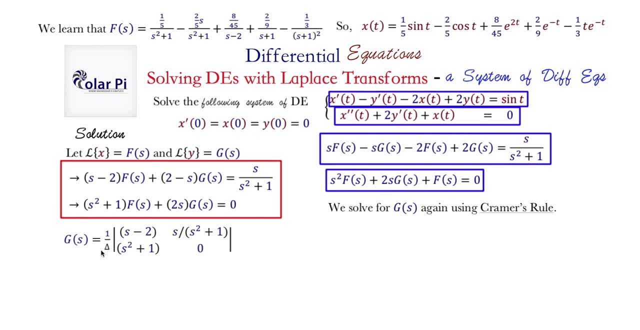 we're solving for uh g, but uh, just as before when we're solving for f, uh, that um determinant of um, two by two matrix of coefficients, right like that's that delta. that delta is in the denominator and it's this uh determinant that's going to be the numerator. 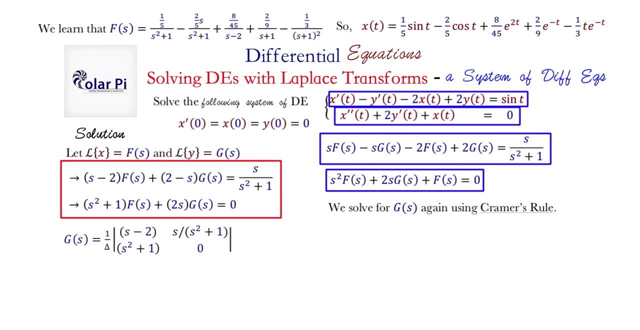 and that's clearly what this math says right there. but just like you know, like, like you know, like wanting to help you out, like it turns out that this determinant, this two by two determinants, simply minus s, and so you have delta downstairs in the denominator, right like, and, if we recall, 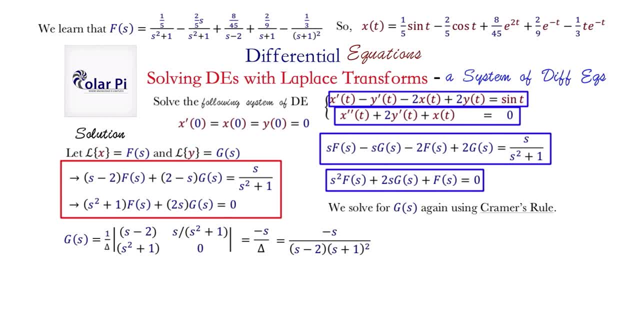 what delta was, which is this. we get to this. this is what g is, and so where to? from here? you named it partial fraction decomposition, right where else? and so then, once you do that, so more fun- you show that this is the same as this here, and then again, once you're here, you need to be able to. 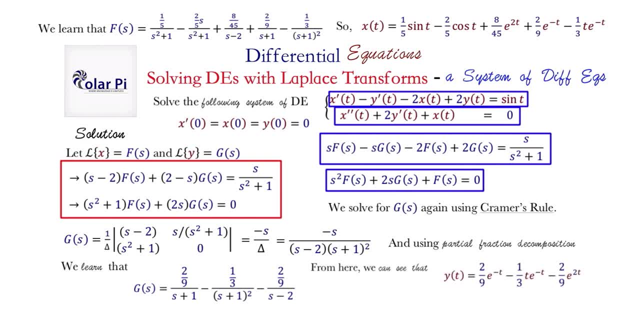 recognize your inverse laplace transforms and, um yeah, things i did in the first video will be helpful. in particular, i highlighted one formula from our good old laplace transform days when we're first studying them. that might be handy when you're going from things like this to this. so check out that first video on solving, uh, differentially. 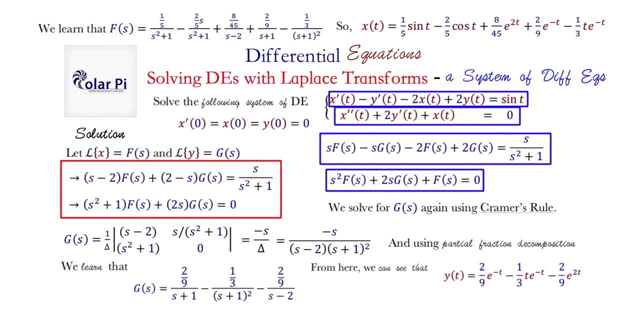 equations. so watch those three examples is basically what i'm preaching, because, well, at this point you've finished watching this. so the only other thing i could have said is watch this video again, which is, well, you know, maybe valuable, so you should do it, but otherwise you.